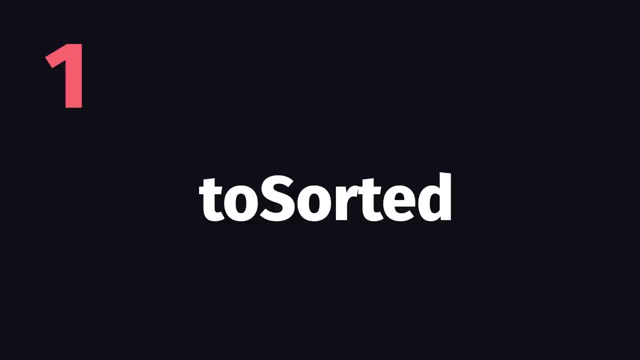 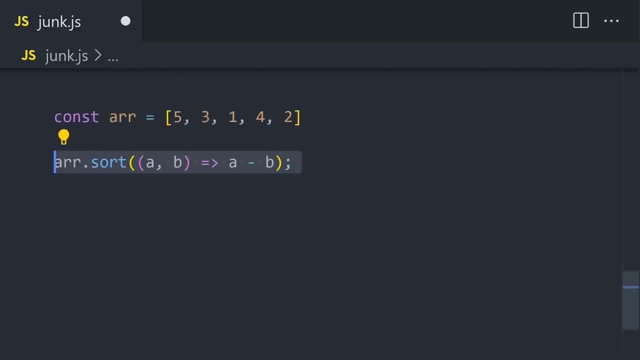 That's a nice little utility, but one I find myself using even more often. One of the new features of JavaScript is array-to-sorted, along with to-spliced and to-reversed. JavaScript already had methods for sort and reversed, but the problem is: 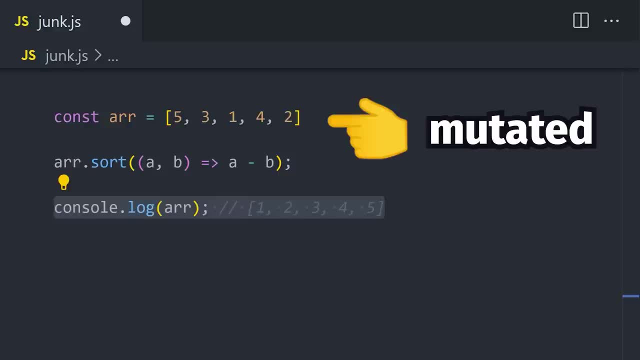 that they mutate the original array in place, And that's confusing, because other methods, like map and filter, don't do that. Instead, they copy the array and return a new one. With these methods, you can now sort, reverse and splice an array by treating the original. 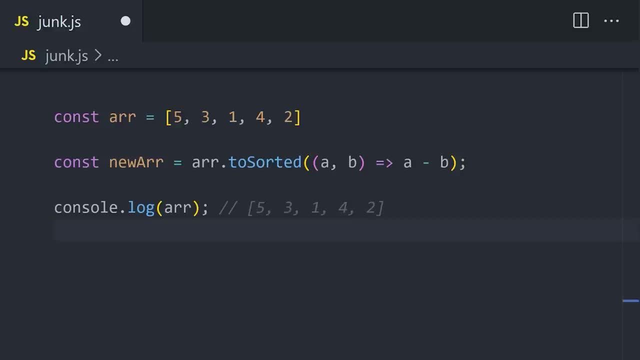 as an immutable value, which tends to be the more sane way to write your code. Web developers also got some cool updates in the form of brand new HTML elements like the search tag is a more semantic way to write your code. You can also use the search tag as a way to. 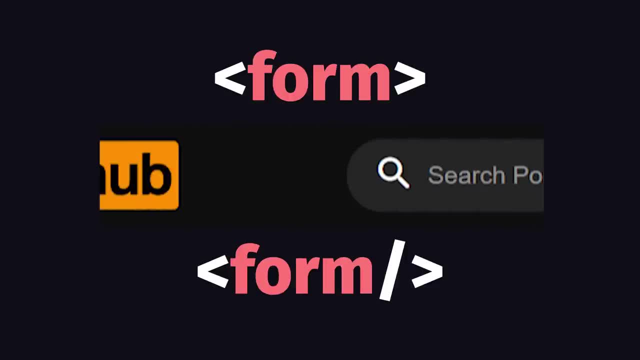 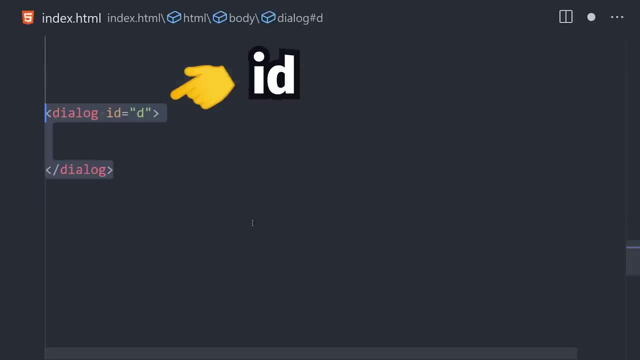 define a search box on a website which can replace the more generic form tag. That's nice, but the dialog element is way more powerful, which allows you to create actual modal dialogs and then control them with JavaScript, using built-in methods like showModal and close. 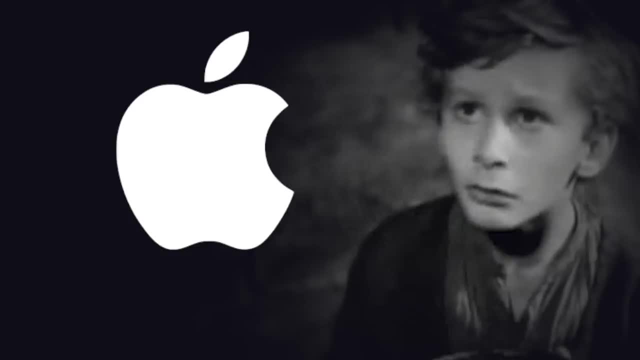 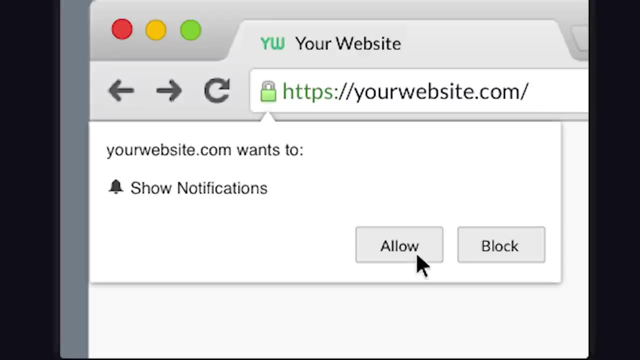 Another nice utility. but that brings us to index 3.. After years of begging and pleading with Apple, iOS finally allows push notifications to come from web apps, And that's a huge win for the .0001% of website users who actually allow websites to send them push notifications. 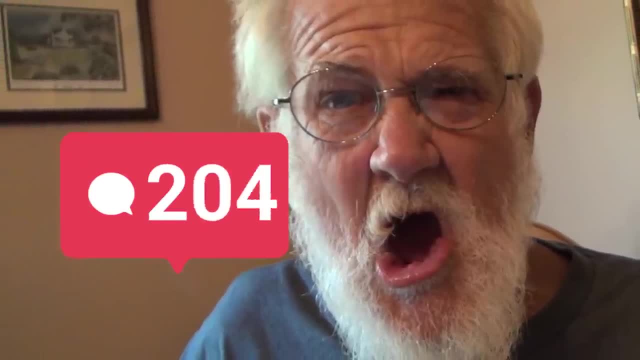 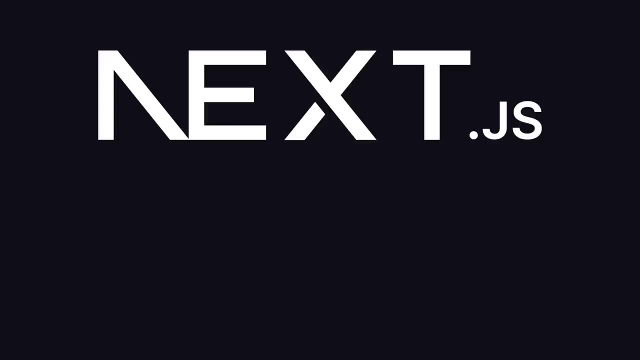 which is most likely your grandpa, who's a native of the US. And now it's time to talk about the fun stuff frameworks. The world's most popular JavaScript framework, Nextjs, is an entirely different framework than it was last year. 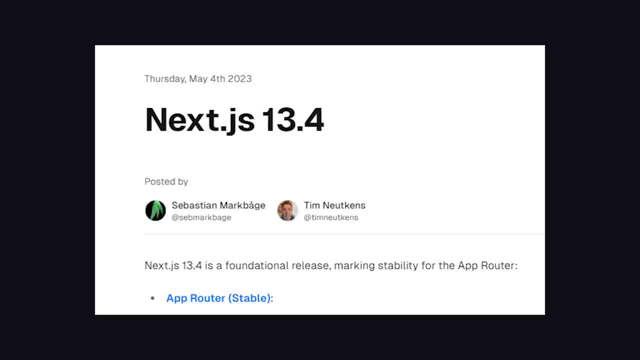 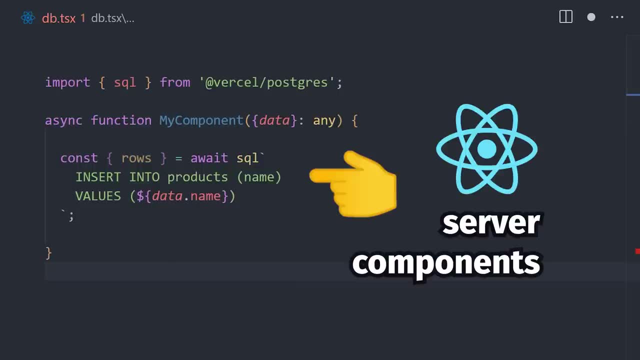 thanks to the app directory, which became stable in May with version 13.4.. The most notable difference is that you can now fetch data directly inside React components thanks to server components, which are React components that can run on the server. The reception. 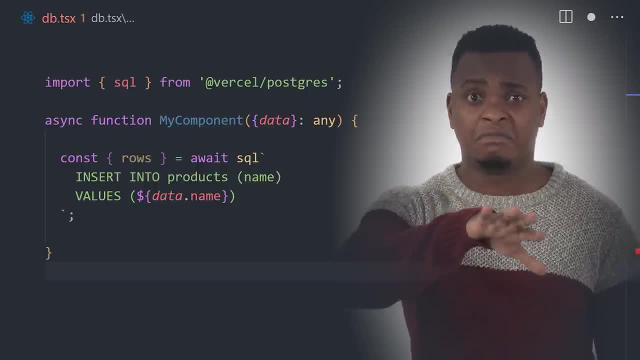 to the app directory has been somewhat mixed. On one hand, it has a lot of awesome new features and can simplify your code, But on the other hand, it has a lot of awesome new features but many have complained about it feeling rushed and half-baked, kind of like the way. 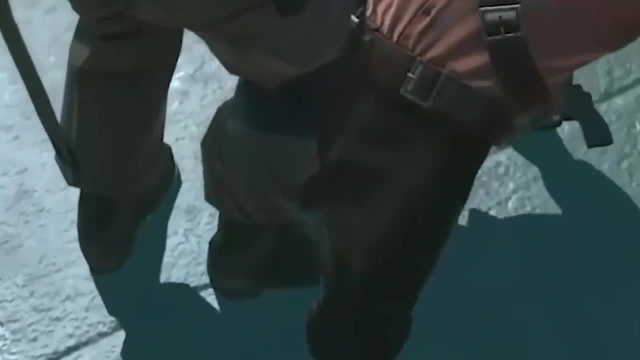 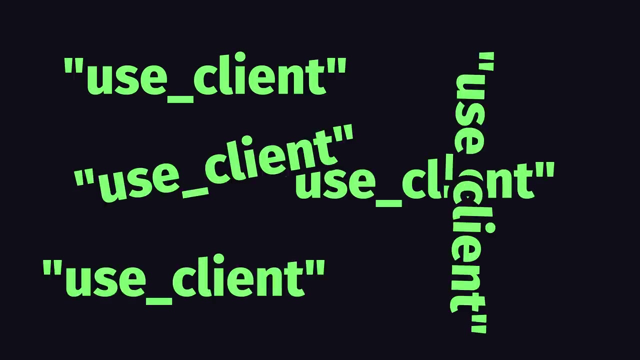 they launch video games nowadays where they just get something out the door then patch it up over the next few years. People have complained about having to use the use client directive everywhere due to breaking existing React libraries. People have complained about the slow dev server which is powered by Rust, which is weird because anything powered by 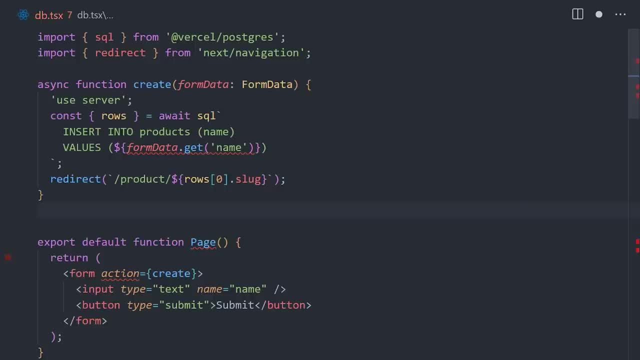 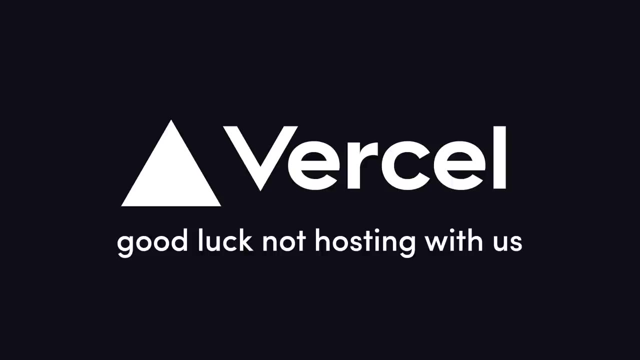 Rust is supposed to be fast And people have compared its new server actions feature to PHP- one of the most offensive slurs you can make against a JavaScript framework. But the biggest issue is that running Nextjs is fairly hard to do correctly outside of Vercel And 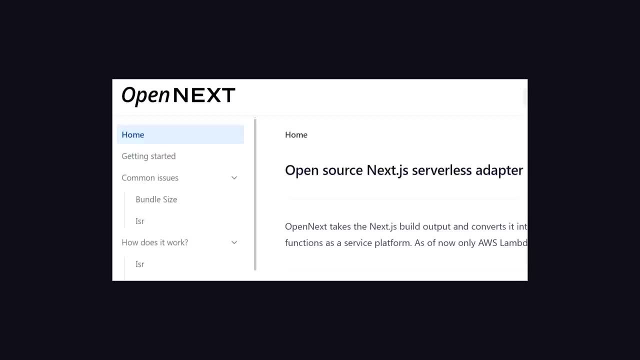 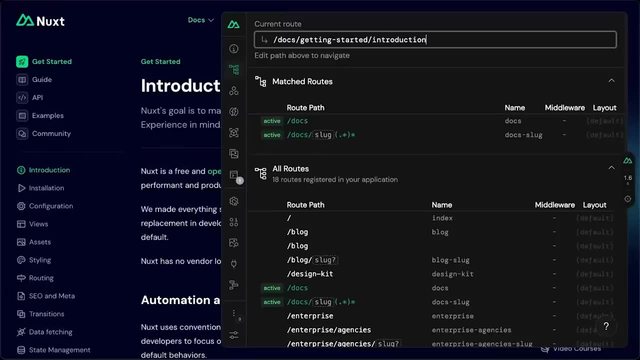 that's led to projects like OpenNext that take on the tedious job of getting it to run anywhere. Nextjs is still the dominant meta-framework, but Nuxtjs and the Vue ecosystem also had a lot of cool updates in 2023, like its dev tools. These tools run directly in. 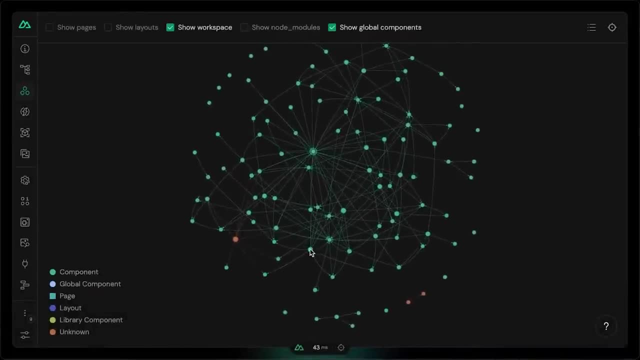 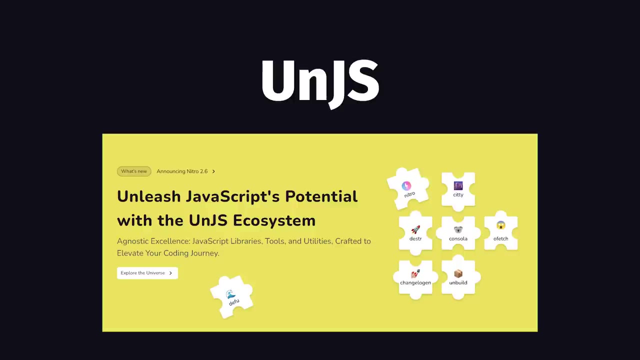 the browser and make it much easier to understand the structure of a complex application. But one thing you may not know about Nuxtjs is that many of its components are available through the unified JavaScript tools ecosystem. Like, if you don't care about Vuejs and just. 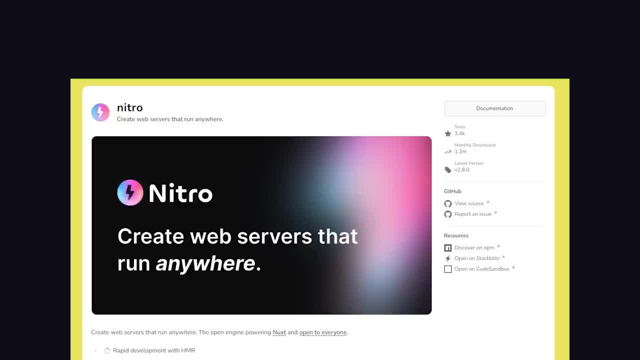 want a web server. you can use Nitro to build a fast server with plain JavaScript. What's funny is I think the Vuejs and Vercel have a lot in common, but I don't think they're the same. The Vuejs ecosystem has changed the least in 2023, and, as a consequence, it feels like 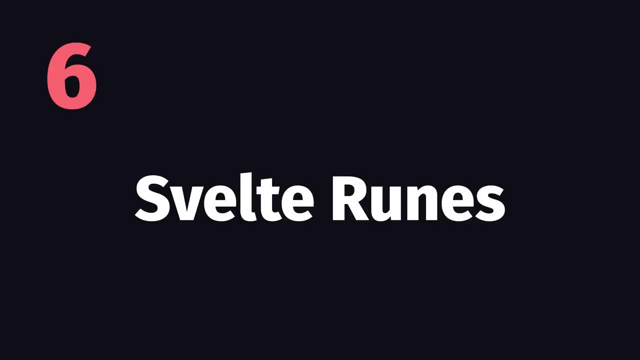 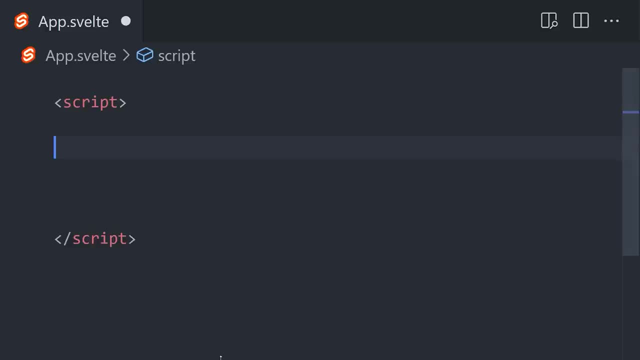 the most stable and predictable ecosystem. Svelte, on the other hand, got runed in 2023.. In a shocking announcement a couple months ago, Svelte announced a new feature called runes that will dramatically change the developer experience in version 5.. Instead of defining 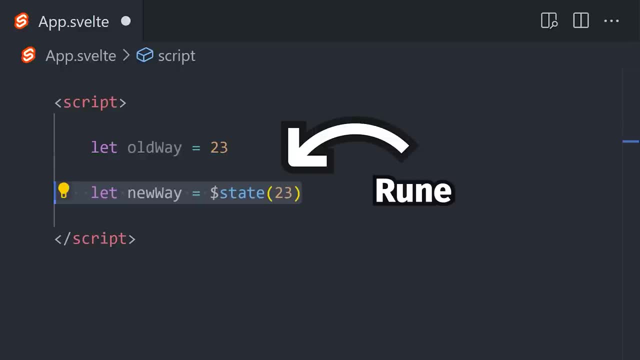 reactive variables with let. there's now this thing called a rune, which is essentially a compiler macro that tells the Svelte compiler this value is reactive. Svelte is also getting rid of the dollar sign, colon syntax and stores with runes like derived and effect. 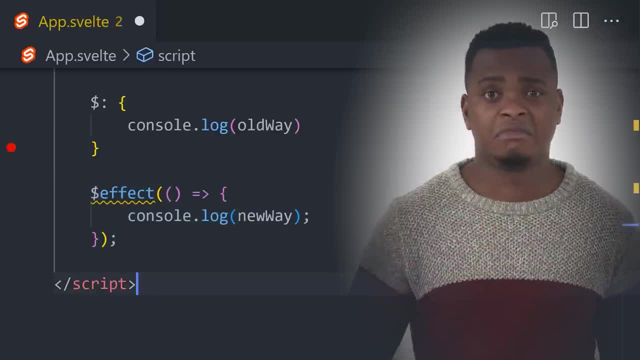 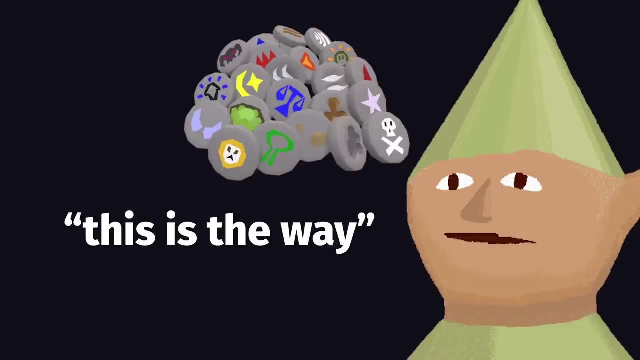 The initial response to these changes were somewhat mixed, with some users feeling like these changes make Svelte look a lot more like React, which is the type of developer experience they're trying to get away from. But, on the other hand, a lot of people love these changes. 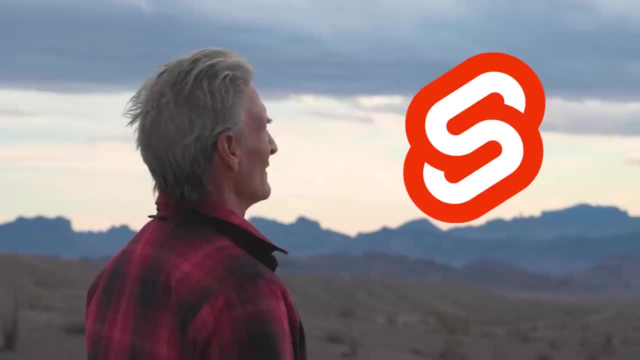 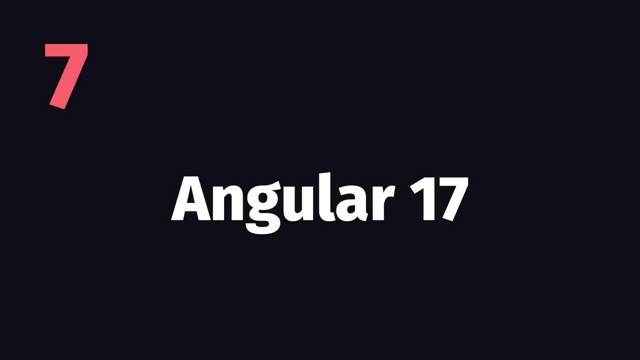 and see them as necessary to evolve the framework in the right direction. As a hardcore user of Svelte myself, I'm waiting for the final release of version 5 before I form an opinion. The award for the most changed framework in 2023,, though, goes to Angular. It has a long 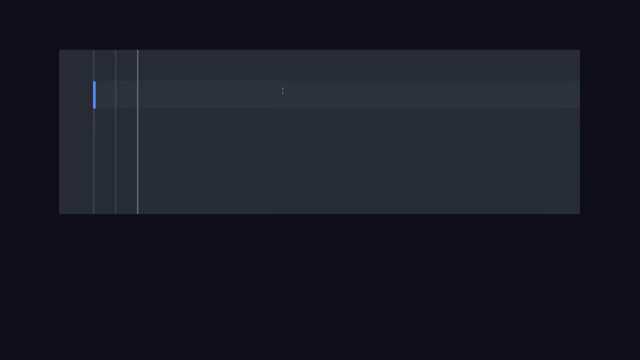 list of new features, but the most notable changes for Angular haters out there would be the new template syntax, which provides a clear view of the framework. The most notable changes include a cleaner way to handle conditionals and loops, replacing things like ngf and ng4. 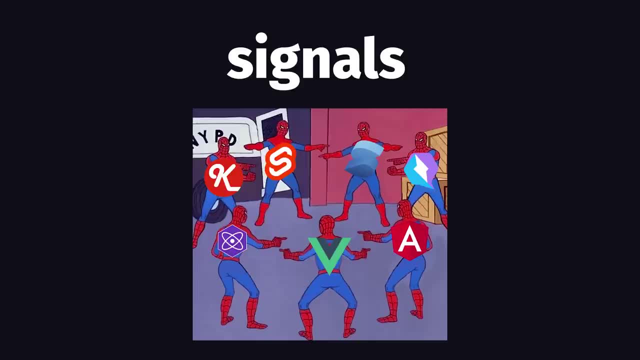 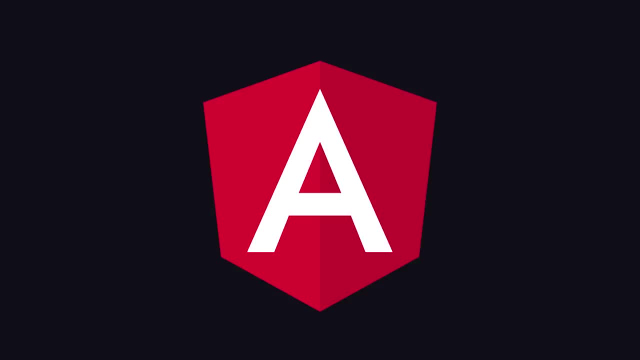 In addition, Angular has also adopted signals, much like all the other frameworks out there, and brings a new feature called deferrable views, which enables declarative lazy loading directly in a template. But, most importantly, Angular has a brand new logo, which was really 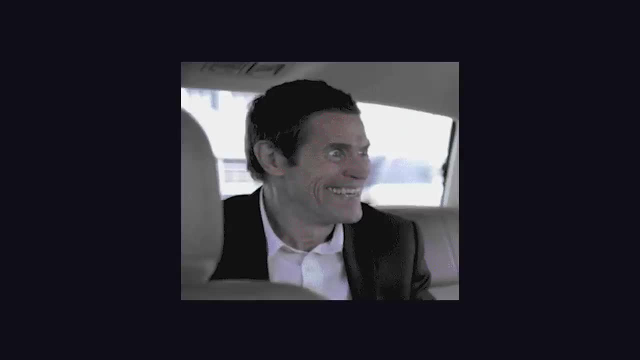 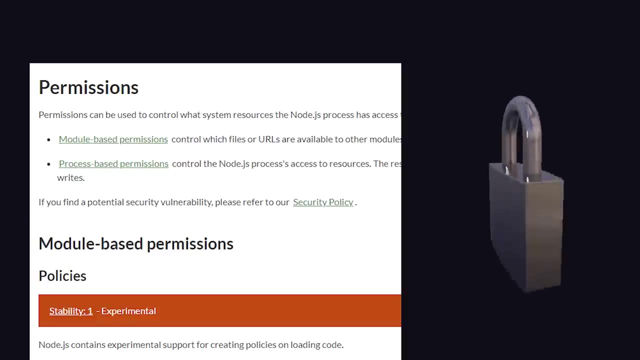 the only thing holding it back from being the world's most popular framework in the past. A lot of crazy changes on the front end, but on the back end, Nodejs has been quietly getting better. With Nodejs version 20, it released a new permissions model, which